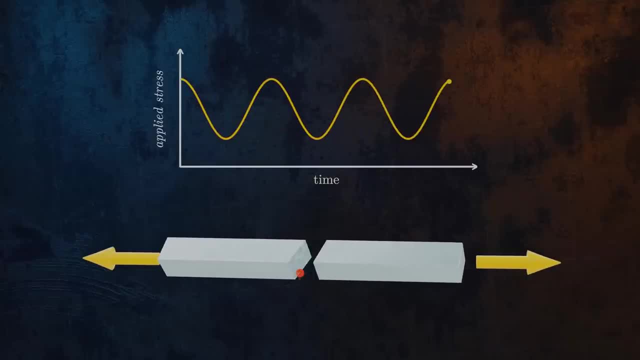 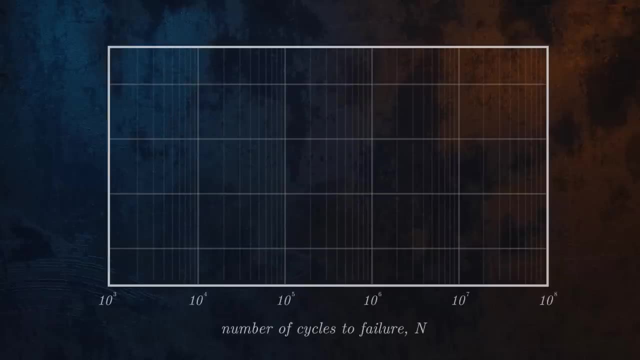 If we repeat this test a large number of times with different applied stress ranges, we can plot the effect of fatigue. Let's start with a graph with the number of cycles to failure- n- on the horizontal axis and the applied stress range- s on the vertical axis. 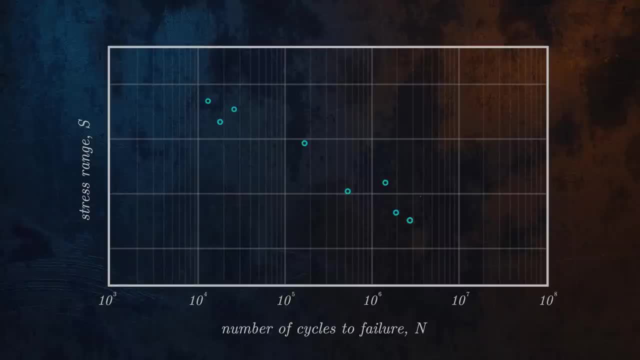 Because the number of cycles to failure can be very large, a log scale is usually used for the horizontal axis. By fitting a curve to the data points, we obtain what is known as an SN curve. The SN curve allows you to calculate the number of cycles until a component is likely to fail for a given stress range. For example, if we have a stress range of N, an alpha value of 4.9 is a variable. For example, if we have an alpha value of 4.9,, an alpha value of 4.9 is a variable. 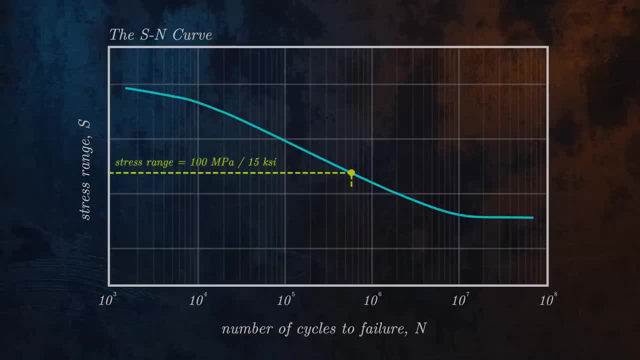 of 100 MPa or 15 ksi. this SN curve tells us that the number of cycles to failure is 500,000.. If we know that our component is subjected to one cycle per minute, we could predict that our component will fail due to fatigue after approximately one year. 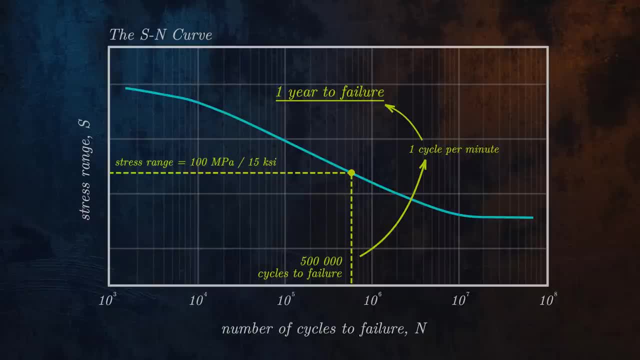 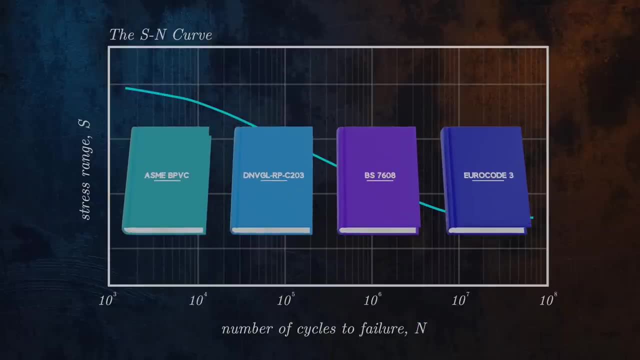 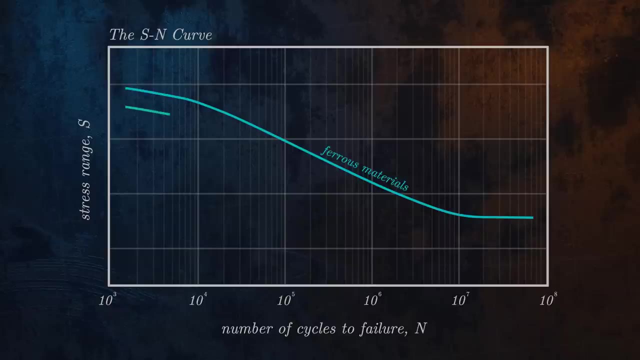 Fortunately, we don't have to perform these time-consuming fatigue tests ourselves. SN curves for many different materials are already published in different engineering codes. For some materials, and in particular for ferrous materials, it is important to note that the SN curve, at a very large number of cycles, becomes a horizontal line. 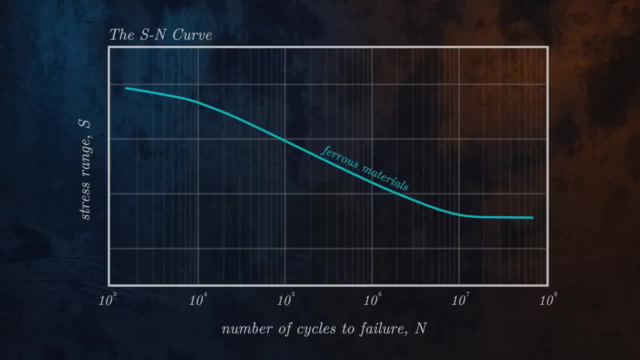 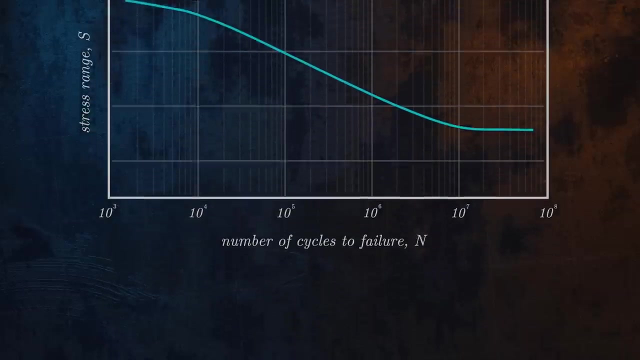 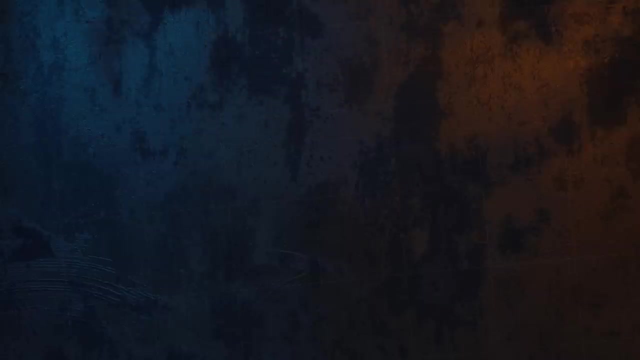 This is known as the endurance limit. Theoretically, the component could be cycled at stress ranges below this level forever, and it will never fail due to fatigue. This makes the endurance limit an important fatigue design parameter. It is common to differentiate between high-cycle and low-cycle fatigue. 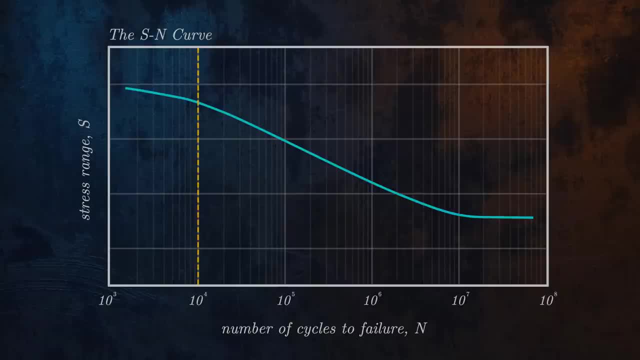 High-cycle fatigue occurs when the applied cyclical stresses are low and failure occurs after a very large number of cycles, typically more than 10,000 cycles. Because the stresses are low, we are only dealing with elastic deformation. Low-cycle fatigue involves higher applied cyclical stresses. 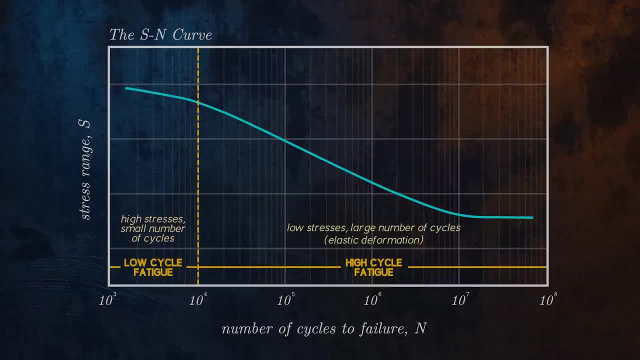 and failure occurs after a very large number of cycles, typically more than 10,000 cycles, Because the stresses involved are above the material's yield stress. both elastic and plastic deformation occur. In these cases, a strain-based approach using, for example, the Coffin-Manson relation. 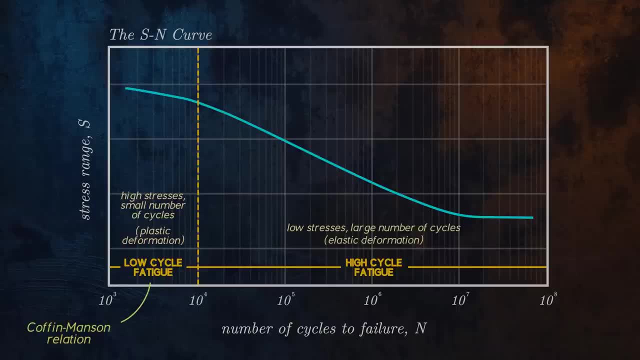 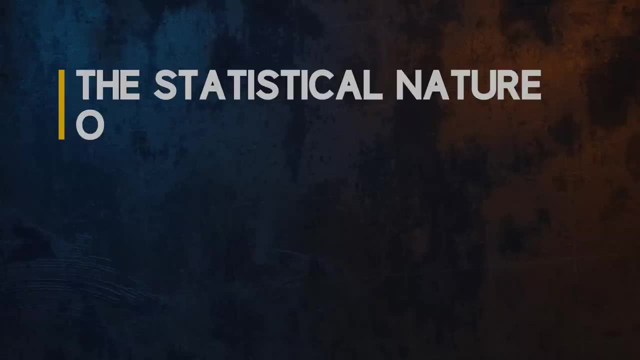 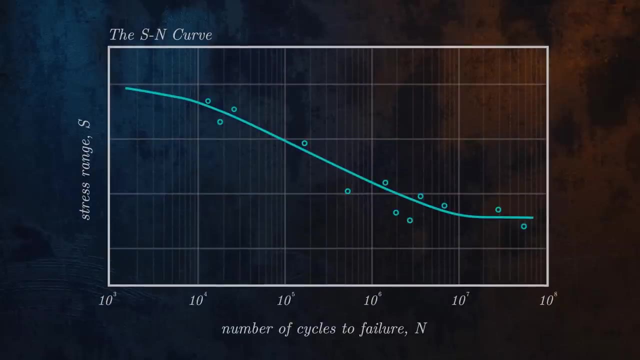 is usually preferred to the SN curve approach. If we return to the data from our fatigue tests, we can see that there is a large amount of stress in the material. We can see that there is a large amount of variability in the data. This is typical for fatigue tests, even when identical test pieces are used. 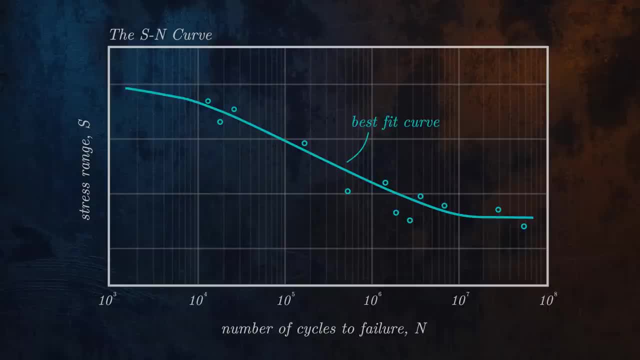 If we use a best-fit SN curve, as we have done here, there is a significant possibility that our component will fail at a much smaller number of cycles than the curve predicts. This test piece, for example, failed at a much lower number of cycles than predicted by our SN curve. 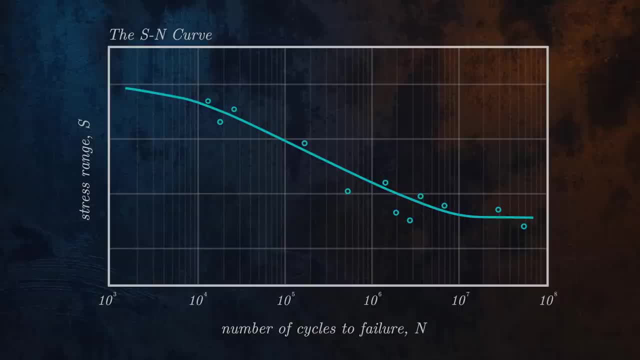 For this reason SN curves published in engineering codes are normally shifted downwards by a certain number of standard deviations to give a reduced probability of failure Here. by shifting the mean curve down on the vertical axis by two standard deviations we have reduced the probability of failure from 50 to 1%. Fatigue tests are usually run for the constant amplitude, fully reversing cycles. you can see here The same stress magnitude is applied in tension and in compression. Let's define a few terms. The stress range is defined as the difference between the maximum and minimum stresses. 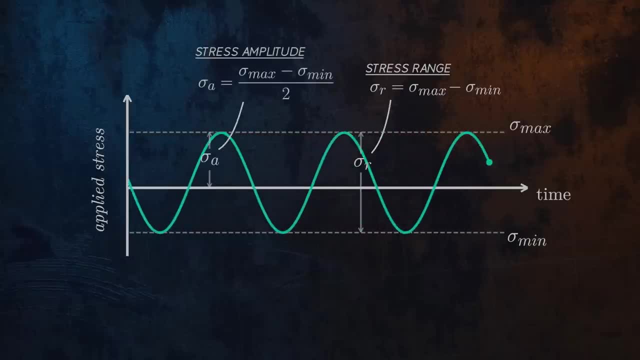 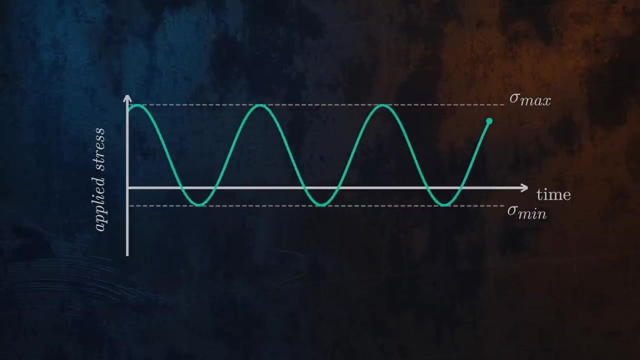 The stress amplitude is defined as half of the stress range. The mean stress is the average of the maximum and minimum stresses. In this case the mean stress is zero. But this is only one very specific type of loading. In some cases we might have a mean stress which is not equal to zero, as shown here. 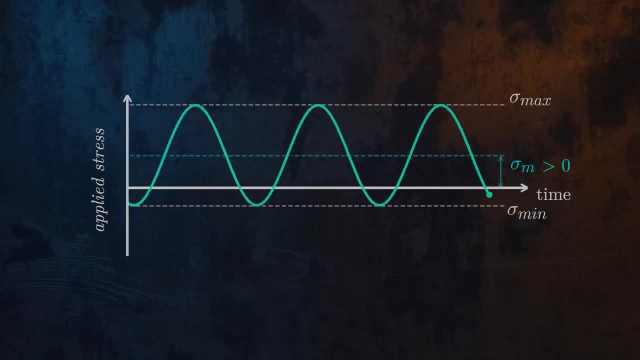 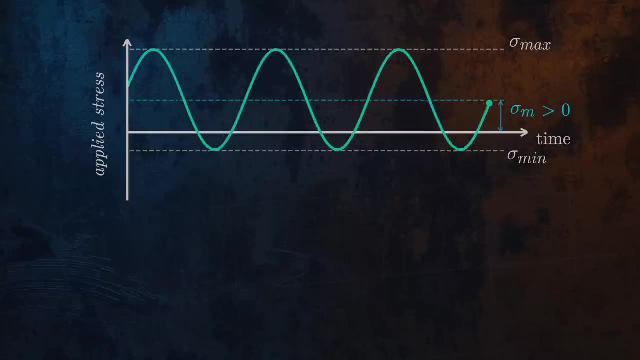 This mean stress will have an effect on the fatigue life. A tensile mean stress will typically result in a shorter fatigue life. One way to account for a tensile mean stress is to use SN curves derived for specific values of mean stress, But these are often not available or would be time-consuming to obtain. 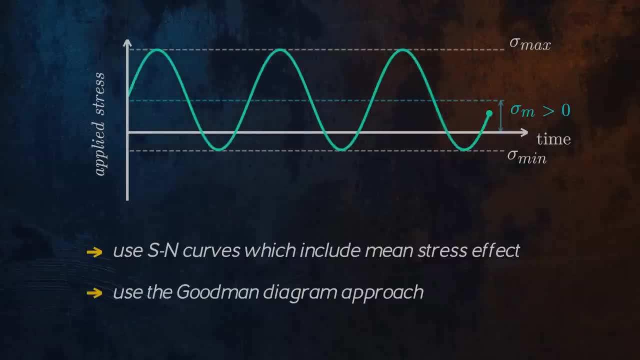 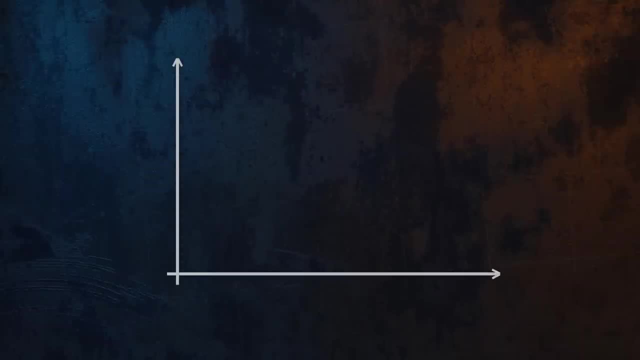 Another approach is to use the Goodman diagram, which adjusts the endurance limit to account for a mean stress. Let's see how it works. On a Goodman diagram, the mean stress is shown on the horizontal axis and the stress amplitude is shown on the vertical axis. 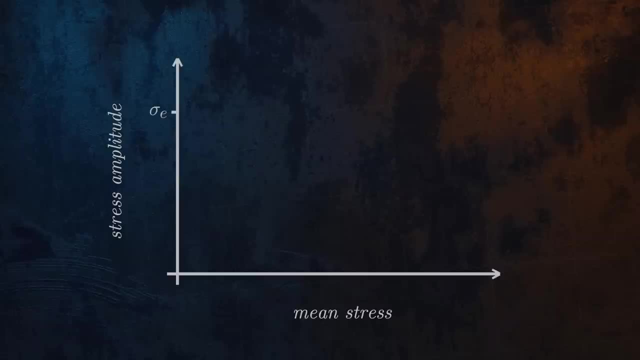 A straight line is drawn between the endurance limit at a mean stress of zero and the material ultimate tensile strength at a stress amplitude of zero. If our cyclic loading conditions are located below the Goodman line, our component will be safe from fatigue failure.